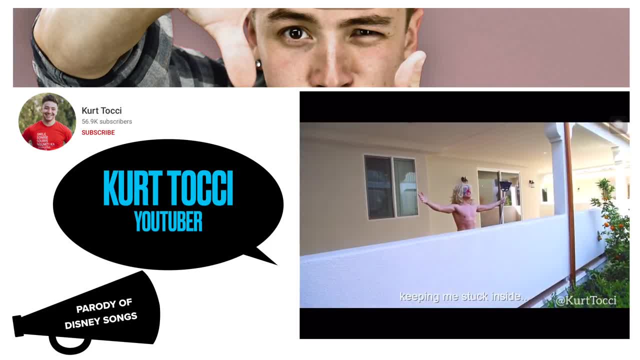 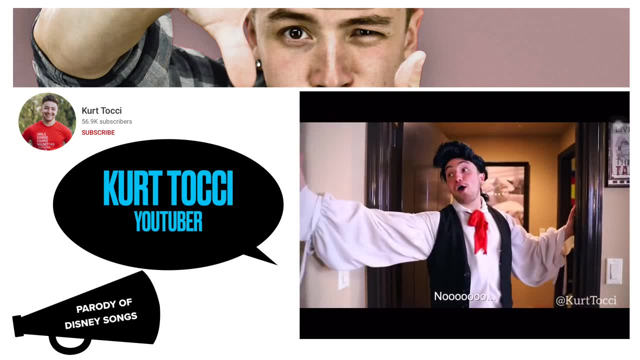 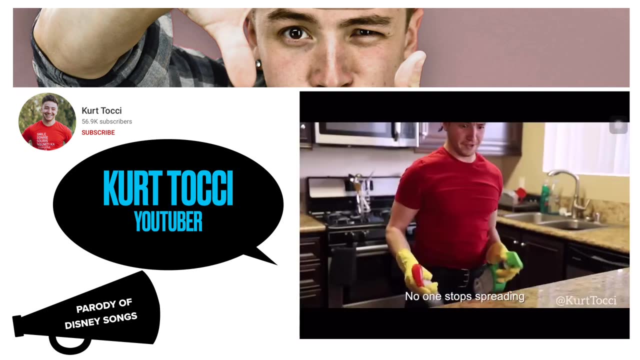 Corona keeping me stuck inside. When will this go all the way? No one clean the floor. Quarantines like Gaston. Quarantines, like Gaston. No one stop spreading COVID-19,. like Gaston, I had a football match today. 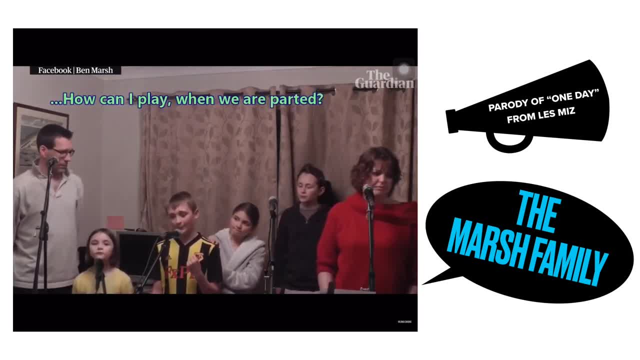 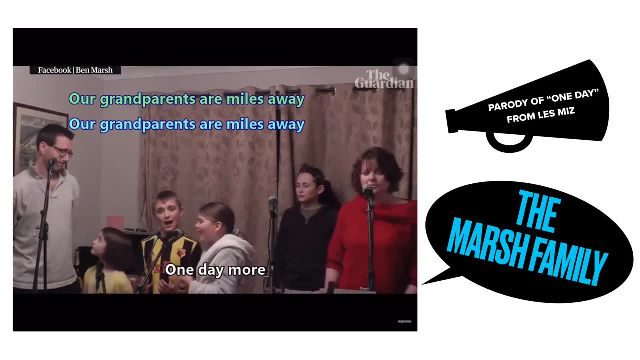 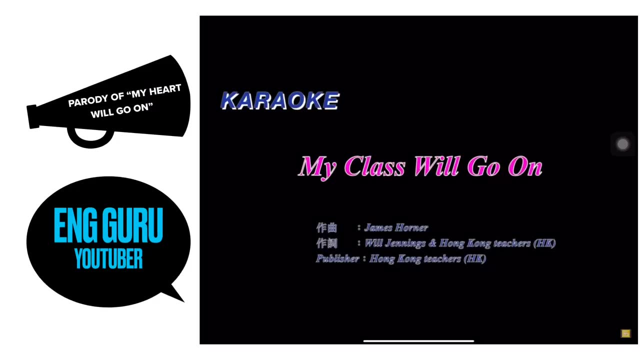 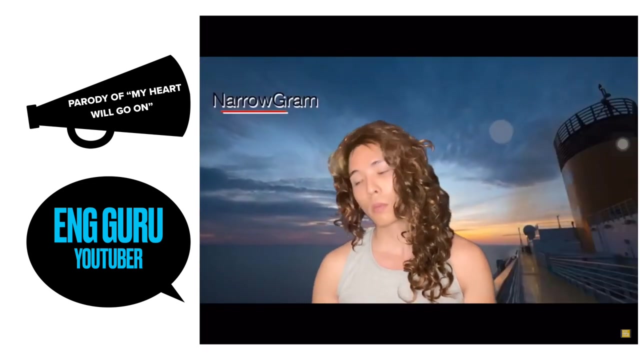 How can I play when we are partying One day more. Our grandparents are miles away. They can't work Skype. we're broken hearts. Let's see how it'll go. That's what they call a study. Will they go to school? 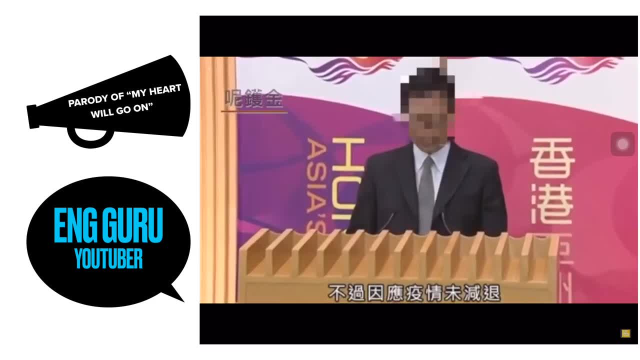 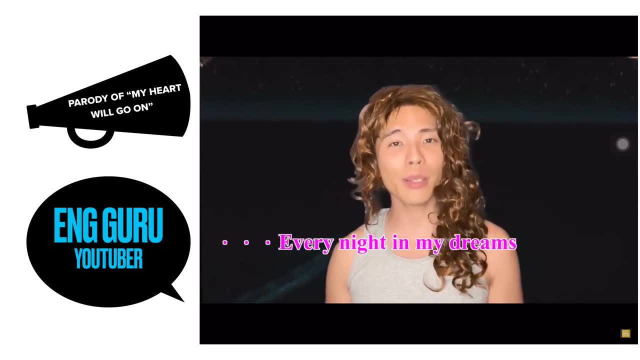 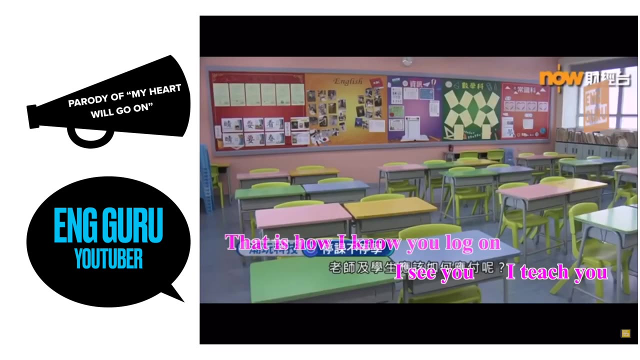 Or this: We have to get back to work. So what can I do? I can't seem to find a job. So what can I do? I have a huge job. I need to find a job here. I'm sure there's something. 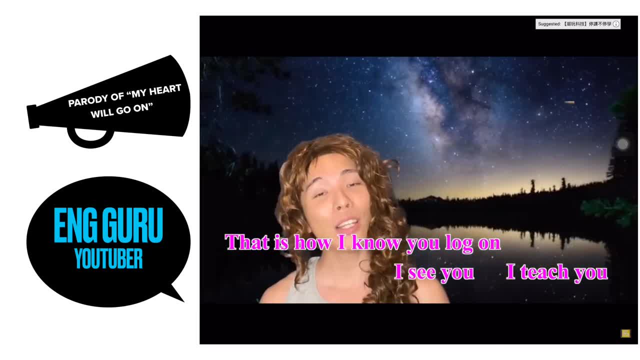 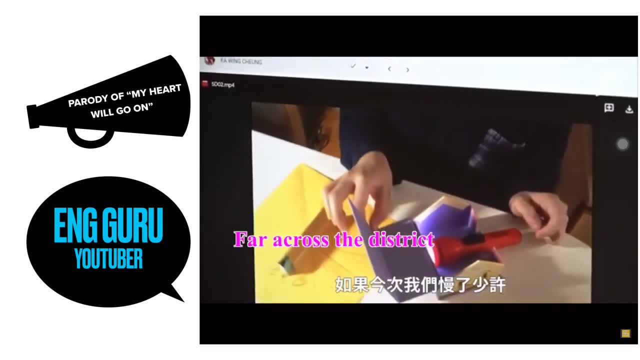 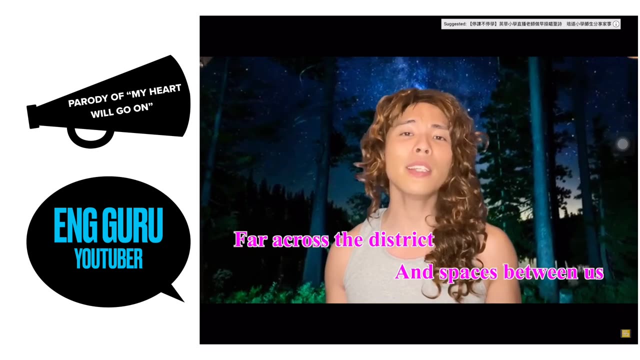 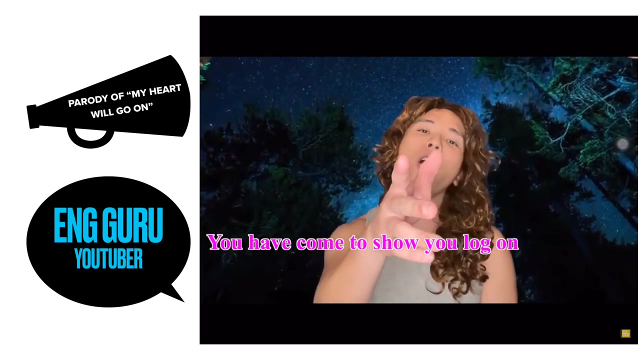 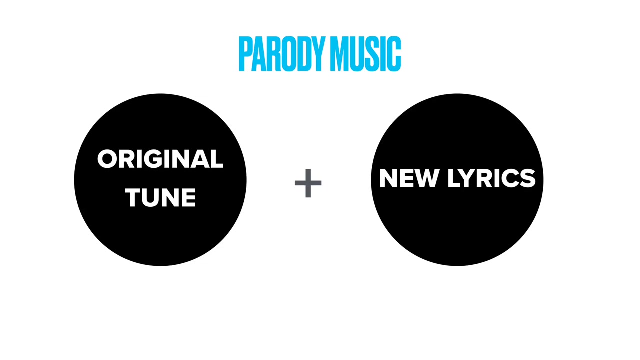 is how I know you logo. Far across the district and spaces between us you have come to show you logo So you can see people are very creative, right, These are parody songs. parody music- Basically they are songs, original ones, sung or written by other singers, songwriters, other bands or groups. 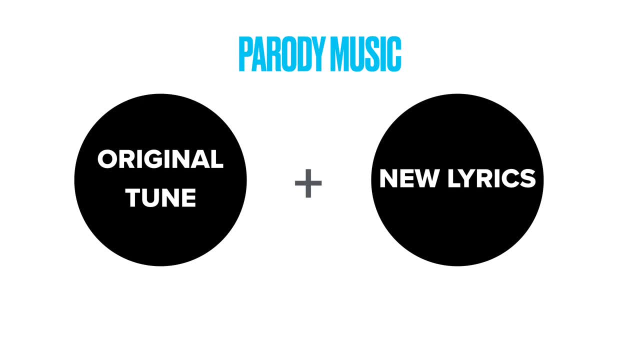 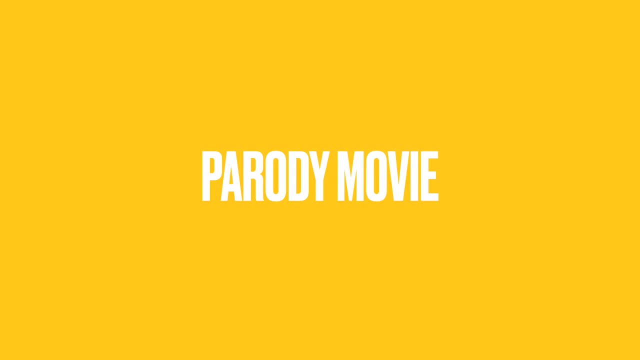 And then you rewrite the lyrics, you create new lyrics for the original songs, And so it becomes a copy of the original song and that is a parody song, a parody music. Apart from parody music, there are different parody movies as well. So when we talk about parody movie, 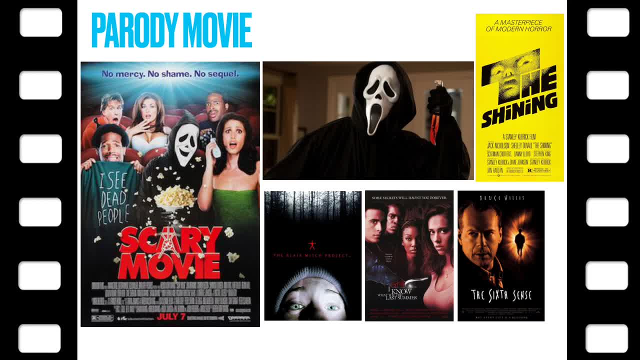 scary movie is definitely the icon of all parody movies Because it's very famous and it has a lot of sequels. And scary movie is a parody movie because inside the movie it has a lot of scenes copied from other very famous scary movies. 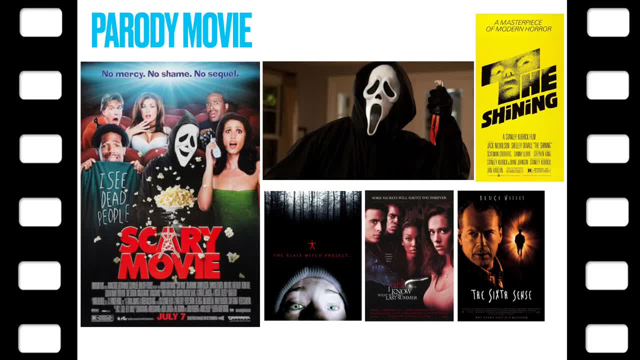 Such as Scream, The Shining- I Know What You Did Last Summer- The Sixth Sense, etc. And scary movie is a comedy movie, So it's to make fun of those original scary movies. So this is the idea of what a parody movie is. 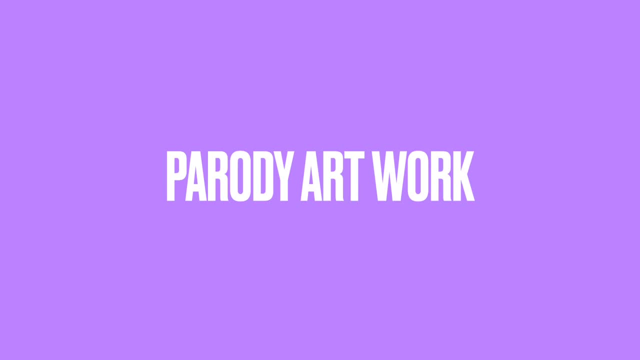 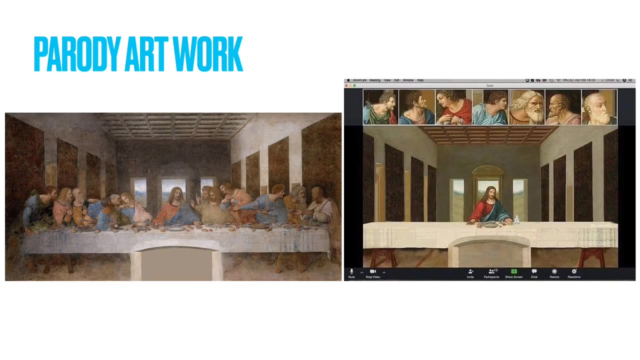 So, apart from parody music, apart from parody movie, there are also pieces of parody artwork. So during this COVID-19 outbreak, the most famous one would be this one: The Last Supper. I think Last Supper has been used a lot in different situations. 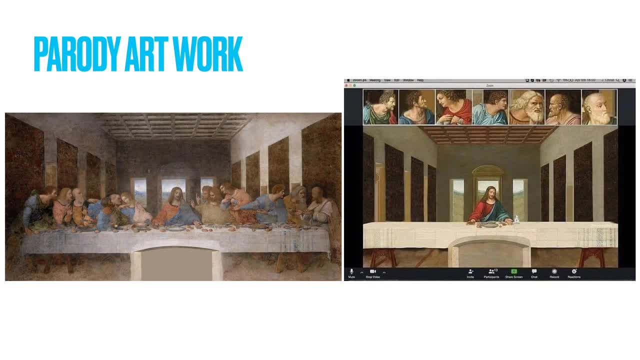 For example, because we need to have social distancing. So even Jesus couldn't have supper with all his apostles And he needs to use video conferencing tool to meet his apostles instead. So this is a parody artwork. The idea is taken from the original piece of artwork. 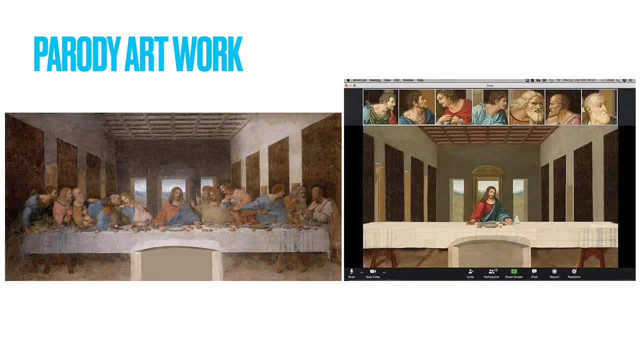 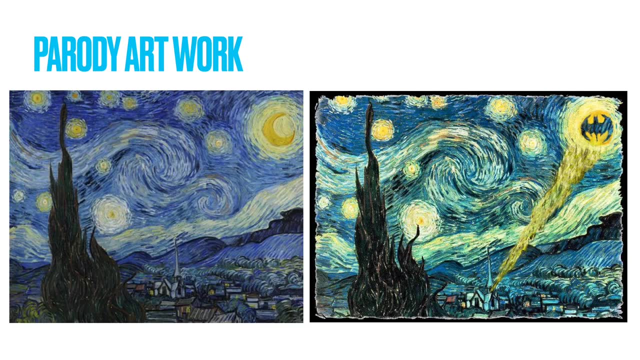 and then added some new elements to it, And it's a copy of the original work, to make fun of it, to give comment and to imitate. So here are two more very famous piece of artwork Like this one: Starry Night. 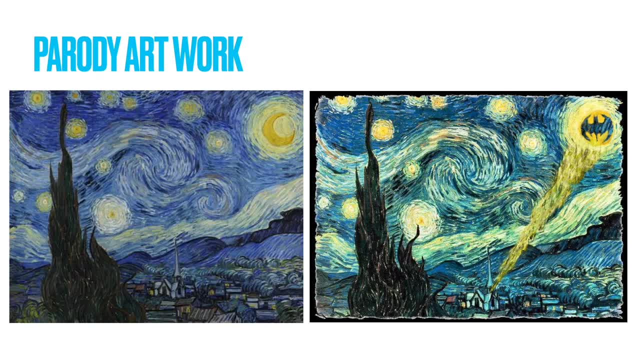 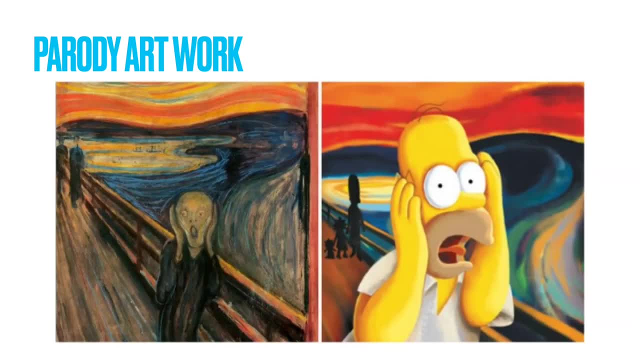 And I really like that- a Batman logo is projected into the sky. So it's like a combination of Gotham City into the Starry Night And this one, The Scream, by a very famous Norwegian artist, Edvard Munch, And there are also a lot of parody artworks based on The Scream. 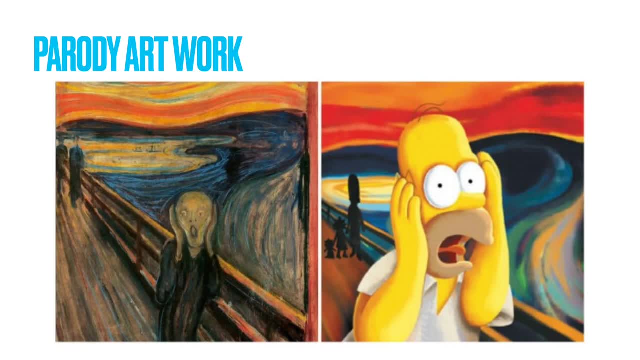 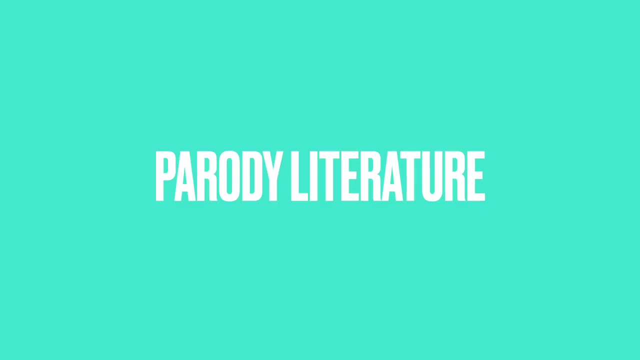 Like this The Simpsons one. So these are some examples of parody artwork. So it's based on the original work and is recreated to imitate, to copy and to make fun or to give comment to the original work. And it's not just music, movie or artwork can be copied. 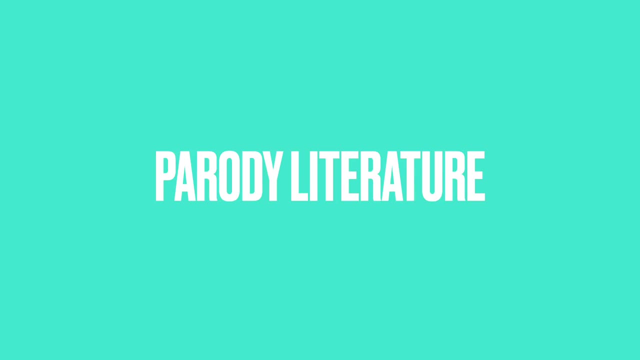 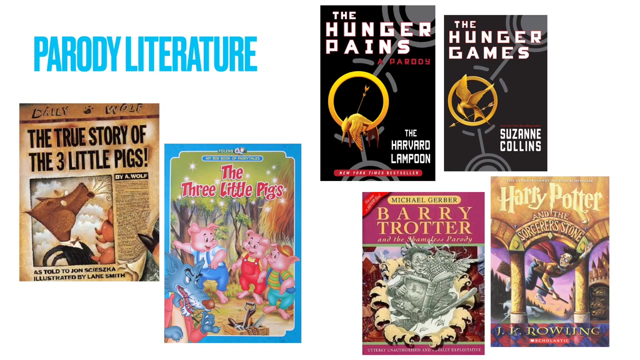 Actually, even literature can be copied as well. So here are some parody literature, Like, for example, The Hungry Pains from The Hunger Games or Barry Trotters from Harry Potter Or The Three Little Pigs, and the parody of it would be.